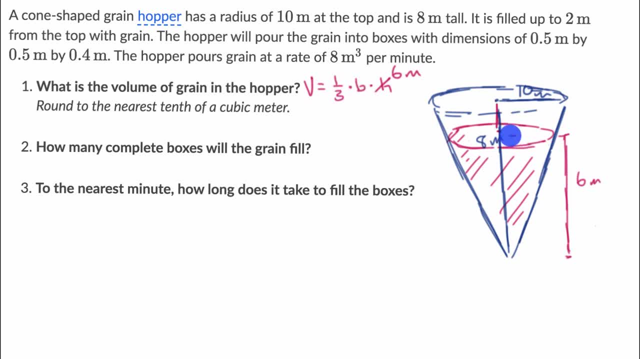 Well, how do we do that? Well, we'd have to figure out the radius of the base. Let's call that R, right over here. And how do we figure that out? Well, we can look at these two triangles that you can see on my screen. 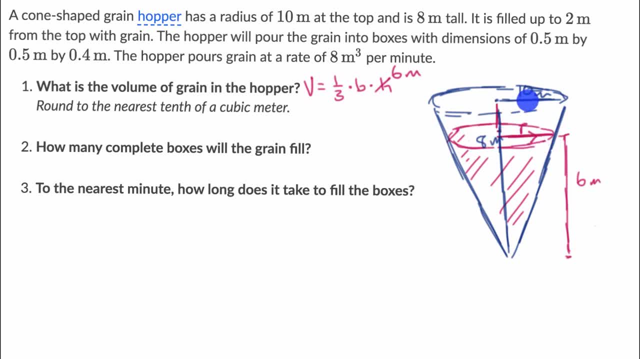 and realize that they are similar triangles. This line is parallel to that line. This is a right angle. This is a right angle because both of these cuts of these surfaces are going to be parallel to the ground, And then this angle is going to be congruent to this angle. 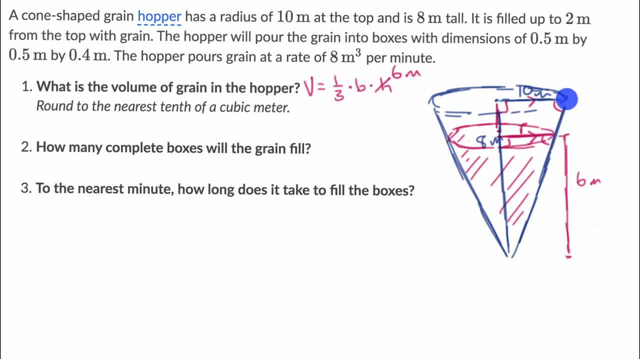 And then this angle is going to be congruent to this angle, Because you could view this line as a transversal between parallel lines and these are corresponding angles, And then both triangles share this, So you have angle, angle, angle. 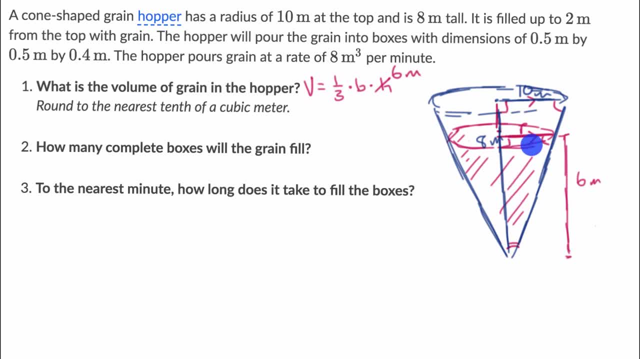 These are similar triangles And so we can set up a proportion here. We can say: the ratio between R and 10 meters- the ratio of R to 10, is equal to the ratio of six to eight, is equal to the ratio of six to eight. 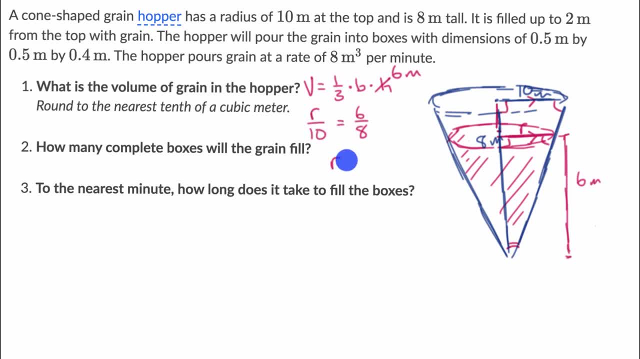 And then we could try to solve for R. R is going to be equal to. R is equal to: multiply both sides by 10,. multiply both sides by 10, and you're going to get 60 over eight. 60 over eight. 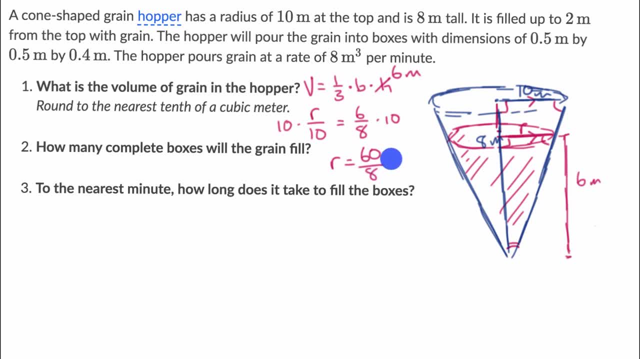 eight goes into 60, seven times, with four left over. So it's seven and four eighths, or it's also 7.5. And so if you want to know the area of the base right over here, if you wanted to know this B. 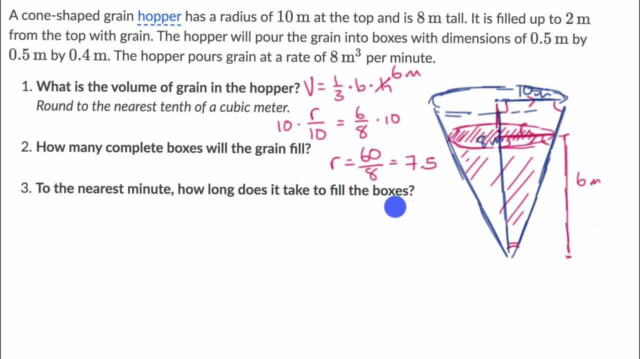 it would be pi times the radius squared. So B in this case is going to be pi times 7.5.. We're dealing with B, We're dealing with meters squared, And so the volume- to answer the first question- the volume is going to be one third. 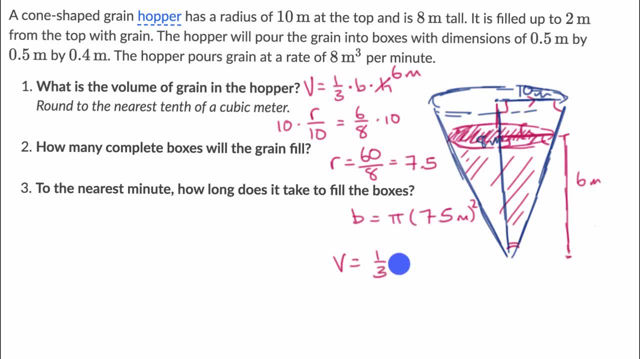 times the area of the base, this area up here, which is pi times 7.5 meters, squared times the height, So times six meters. And let's see, we could simplify this a little bit- Six divided by three or six times one third. 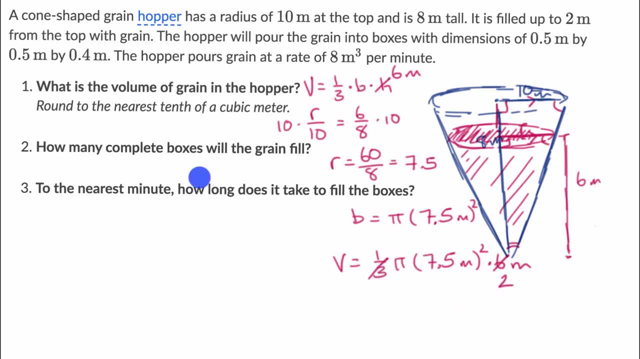 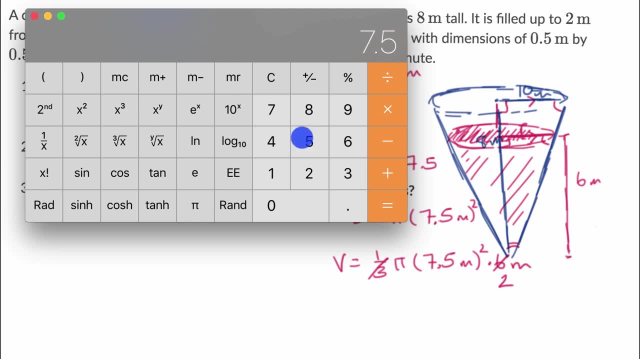 is just going to be equal to two, And so let me get my calculator. They say round to the nearest 10th of a cubic meter. So we have 7.5 squared times two. times pi is equal to if we round to the nearest 10th. 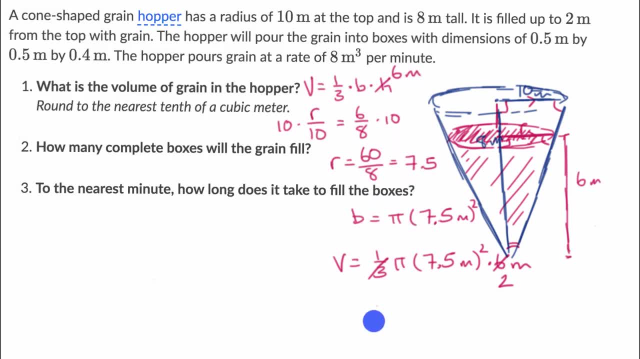 it's going to be 353.4 cubic meters. So the volume is approximately 353.4 cubic meters. So that's the answer to the first part right over there. And then they say: how many complete boxes will the grain fill? 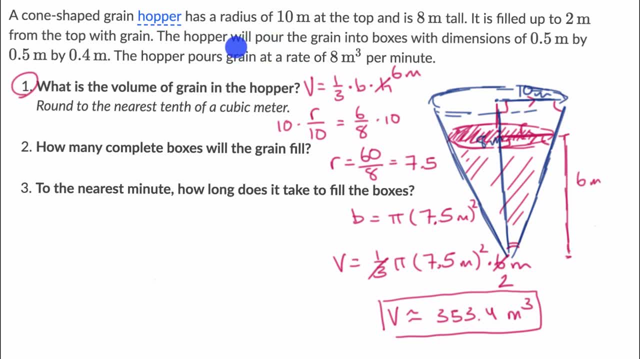 Well, they talk about the boxes. right over here, The hopper will pour the grain into boxes with dimensions of 0.5 meters by 0.5 meters by 0.4 meters. So we can imagine these boxes. They look like this and they are 0.5 meters by 0.4 meters. 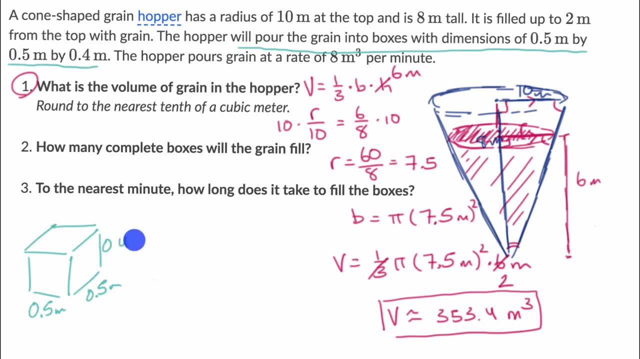 0.5 meters by 0.4 meters. So the volume of each box is just going to be the product of these three numbers. So the volume of each box is going to be the width times the depth times the height. So 0.5 meters times 0.5 meters, times 0.4 meters. 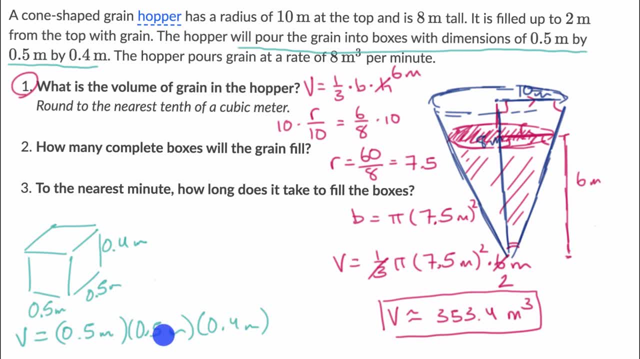 And we should be able to do this in our head, because five times five is 25.. 25 is 0.5.. 25 times four is equal to 100.. But then we have to think. we have one, two, three digits. 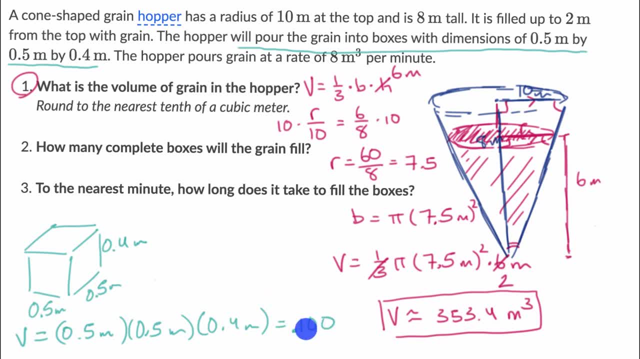 to the right of the decimal point. So one, two, three, So this is going to be a tenth 0.100 cubic meters, So a tenth of a cubic meter. So how many tenths of cubic meters can I fill up with this much grain? 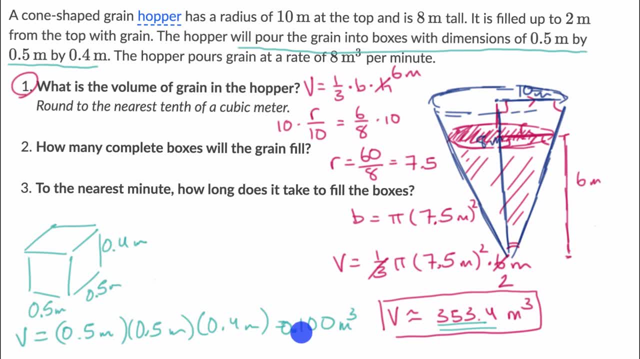 Well, it's just going to be this number divided by a tenth. Well, if you divide by a tenth, that's the same thing as multiplying by 10.. And so, if you multiply this by 10, you're going to get 3,534 boxes. 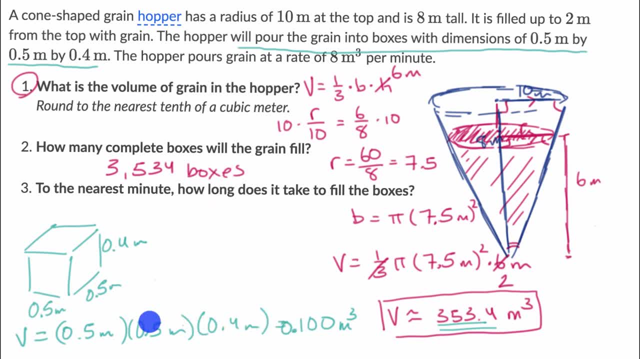 Now, once again, let's just appreciate Every cubic meter. you can fill 10 of these boxes And this is how many cubic meters we have. So if you multiply this by 10, it tells you how many boxes you fill up. 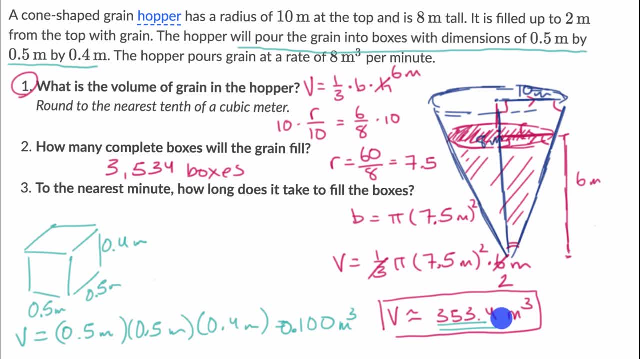 And one way to think about it. we've seen this in other videos. we're shifting the decimal one place over to the right. We're shifting the decimal one place over to the right place, over to the right, to get this many boxes. 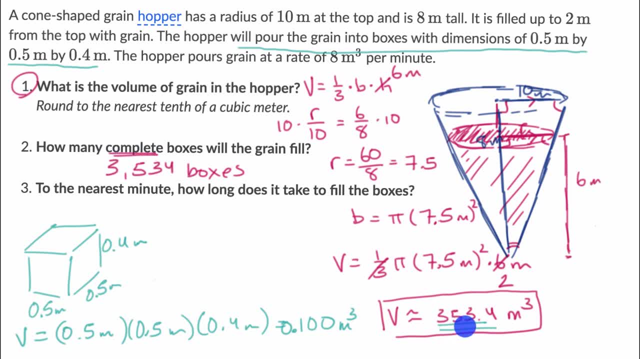 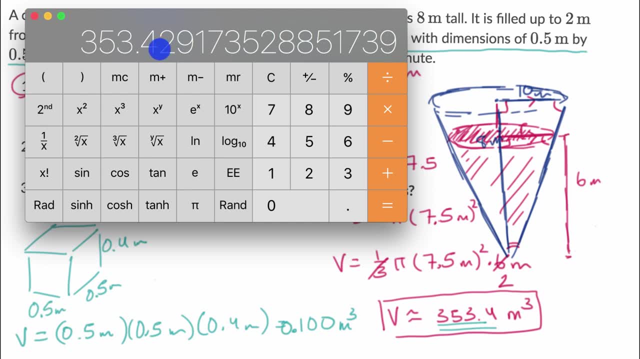 And it's important to realize complete boxes, because when we got to 353.4, we did round down, So we do have that amount, but we're not going to fill up another box with whatever this rounding error that we rounded down from. 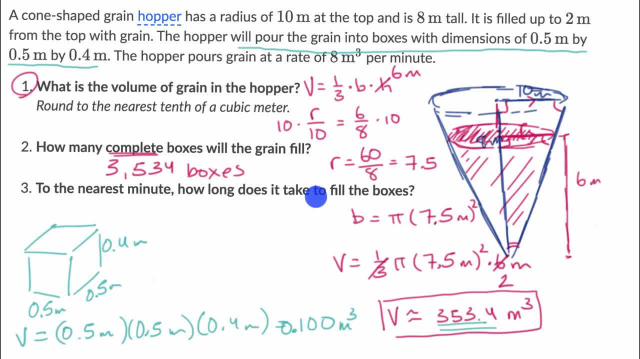 So the last question is, to the nearest minute: how long does it take to fill the boxes? Well, this is the total volume, and we're going to fill eight cubic meters per minute. So the answer over here is going to be our total volume. 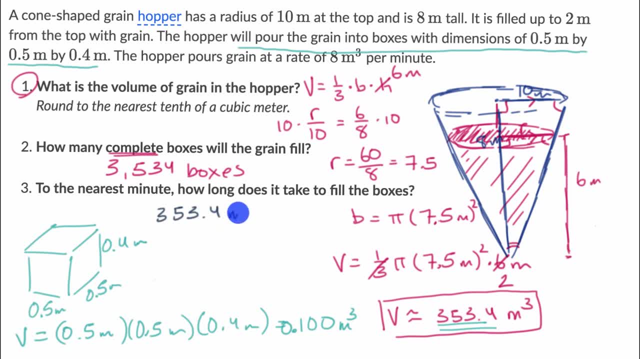 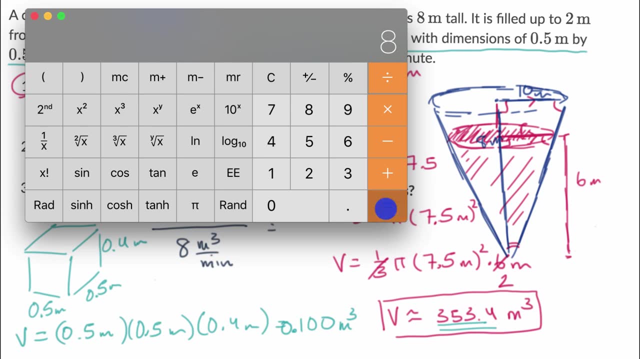 is going to be 353.4 cubic meters And we're going to divide that by our rate, eight cubic meters per minute- And that is going to give us 353.4. divided by eight is equal to, and, if we want to round, 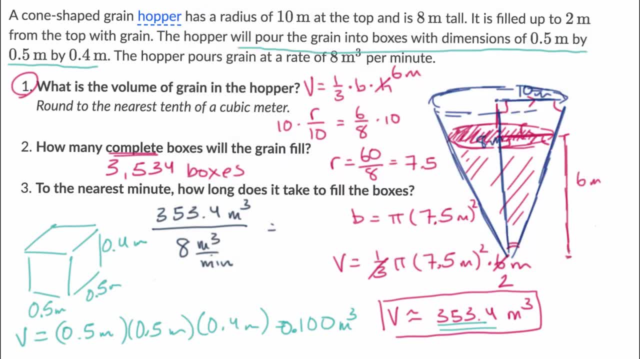 to this number the nearest minute. 44 minutes is equal to approximately 44 minutes to fill all the boxes And we're done. How old is the Earth? Well, by counting the number of isotopes in a sample of rock that's undergone radioactive decay, geologists have estimated the Earth's birthday when it first formed from a solar nebula to be 4.6 billion years ago. But just how long is that, really?